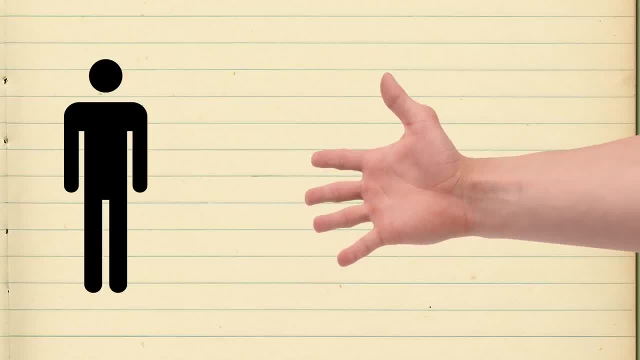 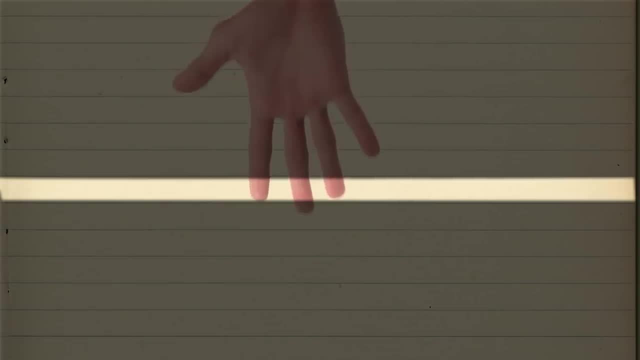 they will see the tip of your fingers appearing, then the rest of your hand slowly coming in. They would constantly see only an infinitely small division of your hand corresponding to their one-dimensional line of sight. Those beings would think of your hand as a shape-changing. 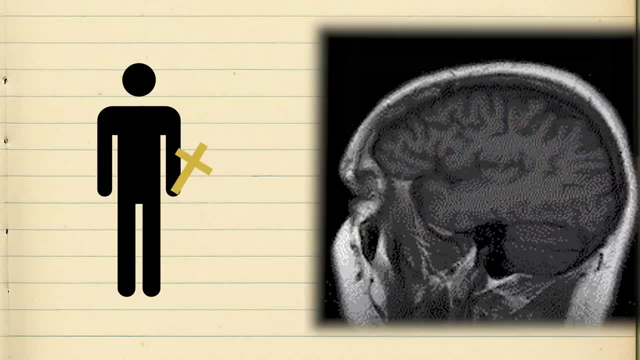 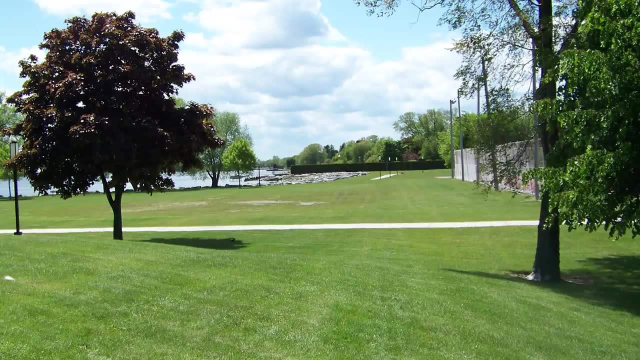 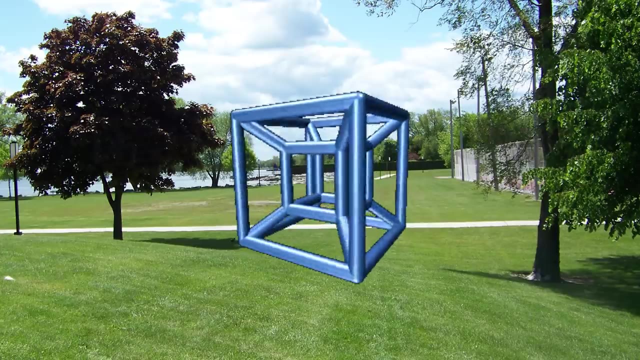 two-dimensional object, Just as an MRI scan views your brain. Now imagine that someone from the fourth dimension comes to our three-dimensional space and puts his hand through. Let's say it's not a hand, but a tesseract- As it would pass through our 3D space. we would see. 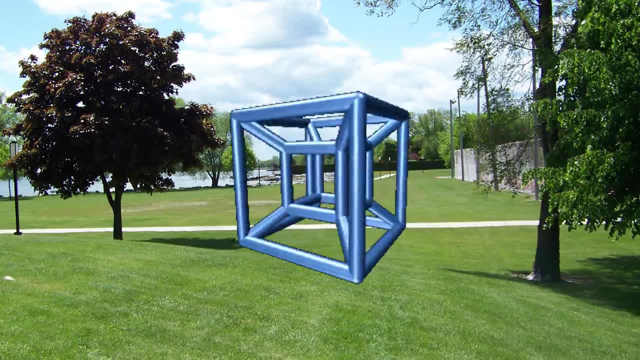 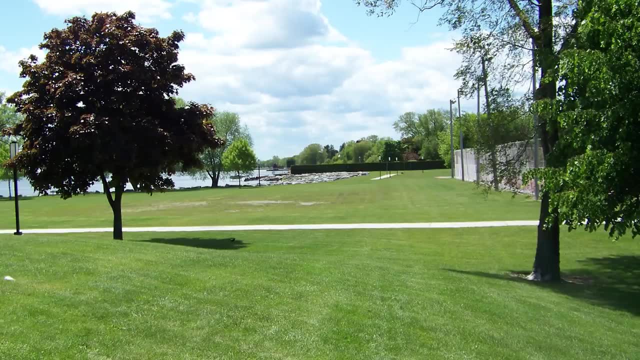 its shape, changing just like our hand did, but in a different way. It gets even more awesome if we consider that time is the fourth dimension, Then the 4D object would be able to control his time. If he were a living being, he could change his age at will, just as we could move. 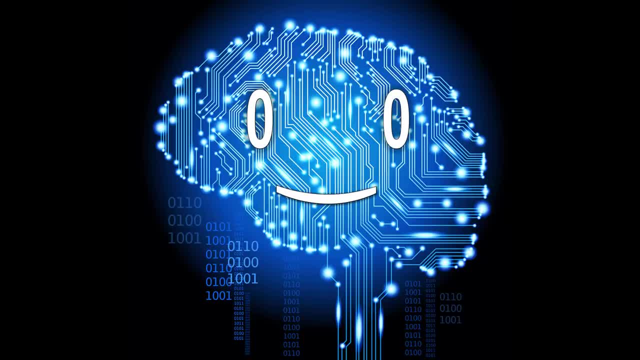 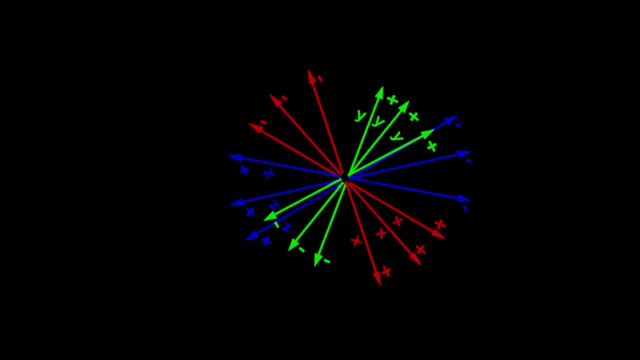 our hand through the two-dimensional world at will. Ok, but let's get back into our own universe. Remember I said that it has more than three dimensions And probably a lot more. The M-theory, which unifies all the super string theories, says that our universe. 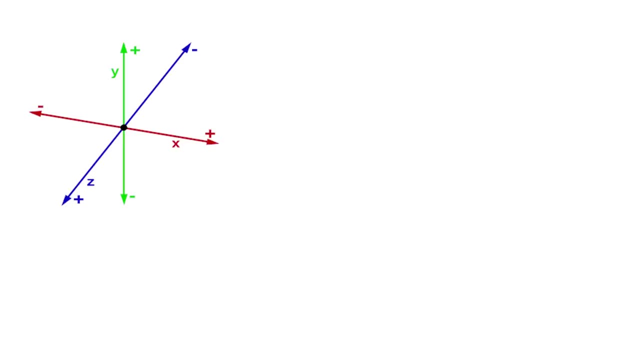 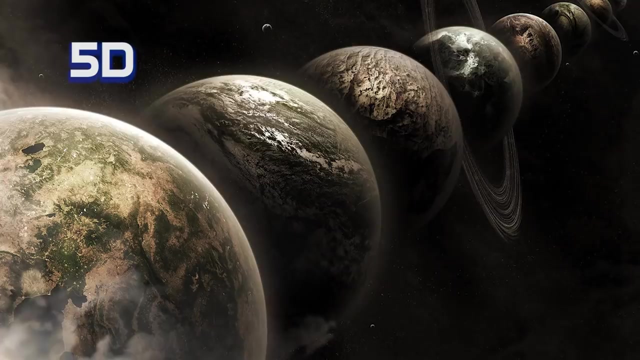 is made up of three spatial dimensions that we are all familiar with: one time dimension and six more small spatial dimensions. According to the string theory, these six additional dimensions would have very interesting properties. If we count the fourth dimension being the time, then the fifth dimension would allow us to travel. 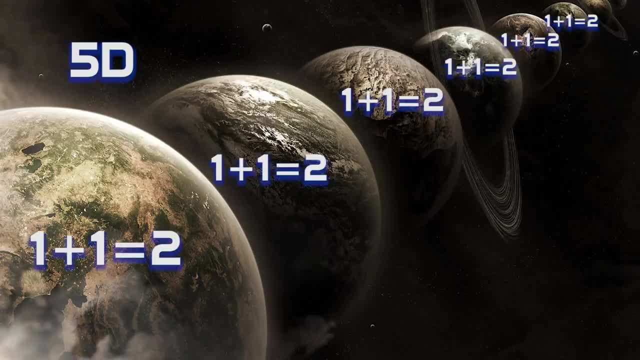 through all the parallel universes that had the same initial coordinates as ours. The sixth one would allow us to travel in time in any of those universes. In the seventh dimension, you could travel to any possible world no matter of their initial coordinates. In the eighth, we could travel 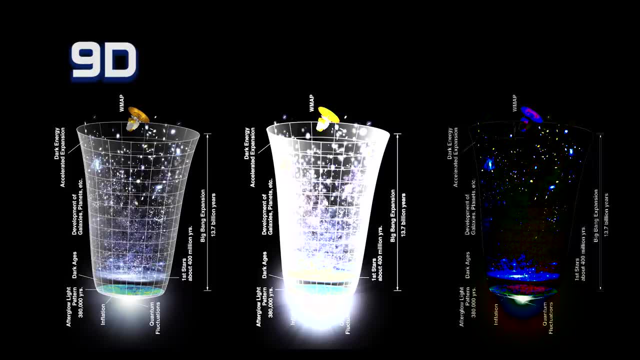 in time in all those universes. In the ninth dimension we can compare all the possible universe histories, starting with all the different possible laws of physics and initial conditions. In the tenth and final dimension we arrive at the point in which everything possible. 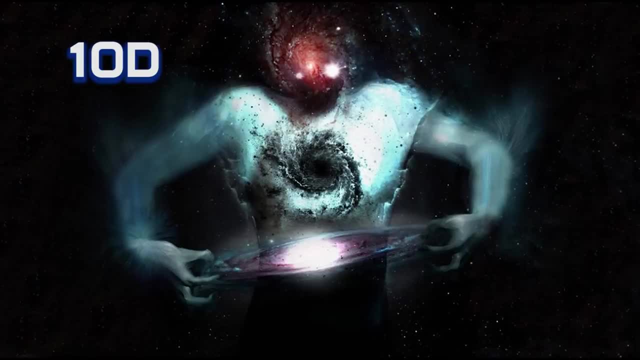 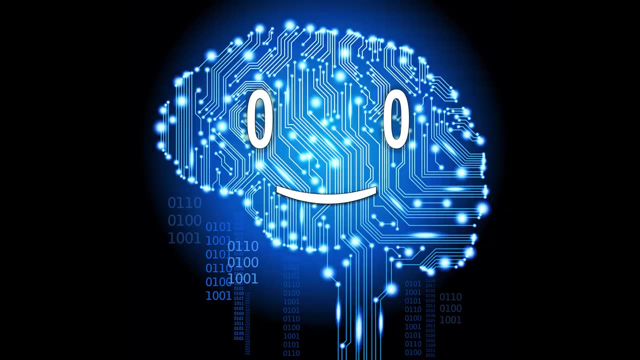 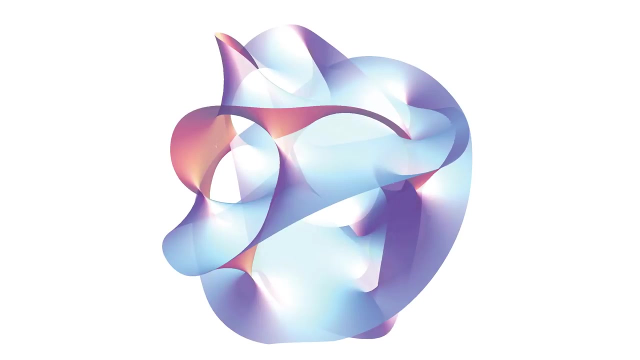 and imaginable is covered. Beyond this, nothing can be imagined by you mortals, which makes it the natural limitation of what we can conceive in terms of dimensions. I swear I didn't make this up, But where are they and why can't we observe any of these dimensions? 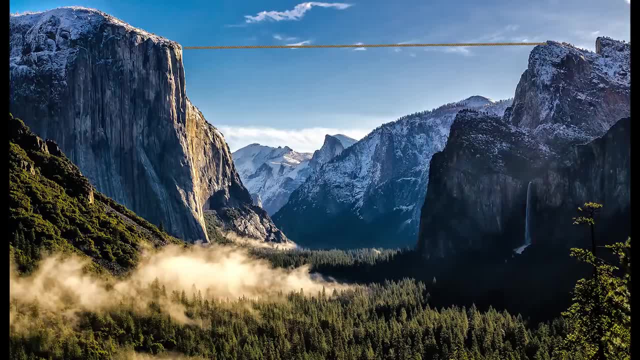 Imagine they're all the same. Imagine they're all the same. There is a very long rope stretched between two mountains. You sit one kilometer away from it and you know there is an ant walking on the rope. Because of the very long distance, 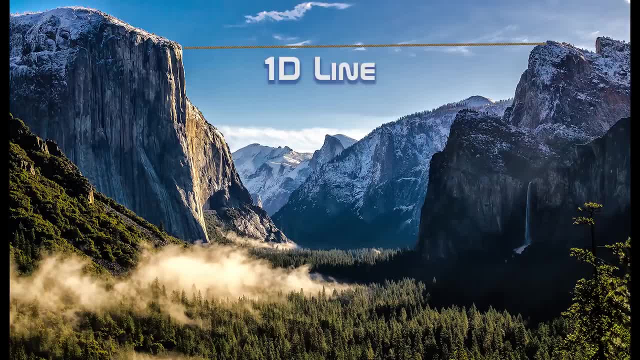 the rope seems to be a one-dimensional line with only length, as its width would be unnoticeable. If you were asked to give the ants coordinates on the rope, you would be able to say: only one piece of data, the distance between the ant and the end of the rope. But in reality, 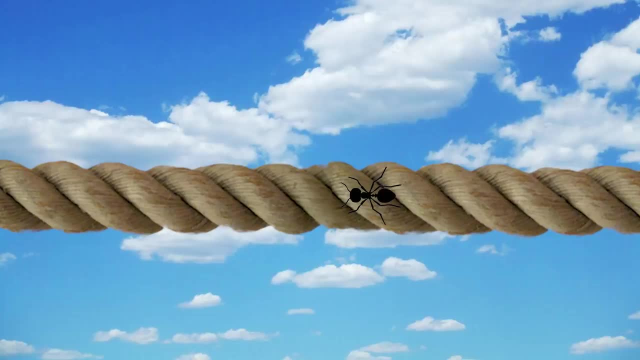 we know that the rope does have thickness, even though it is hard to see from one kilometer away. Take a pair of binoculars and you will observe the second and third dimensions of the rope. The same thing goes for the other six spatial dimensions in our 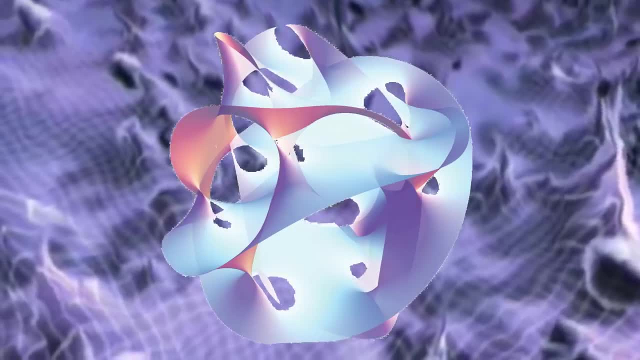 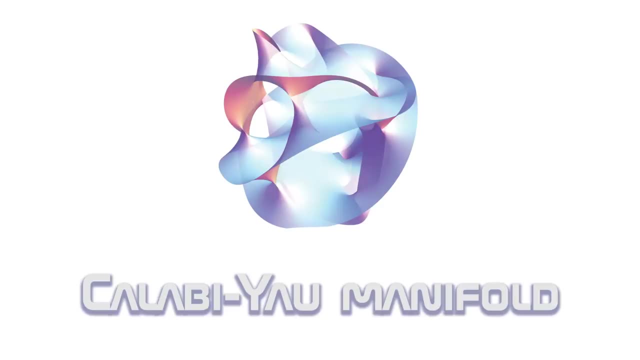 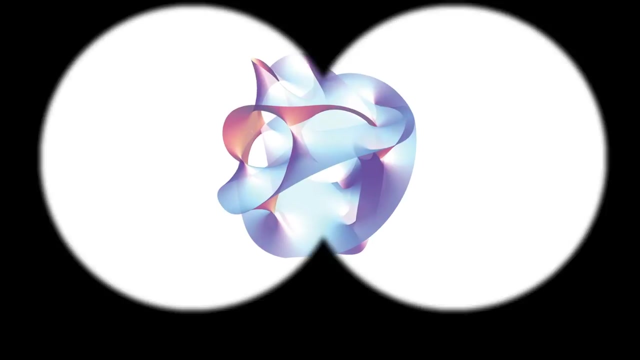 universe. They are on such a small scale that they are indistinguishable from the normal three dimensions. These extra dimensions can be represented in form of a Calabio manifold. I don't know what the f**k is this. don't ask me to explain it. But again, why don't we simply take a 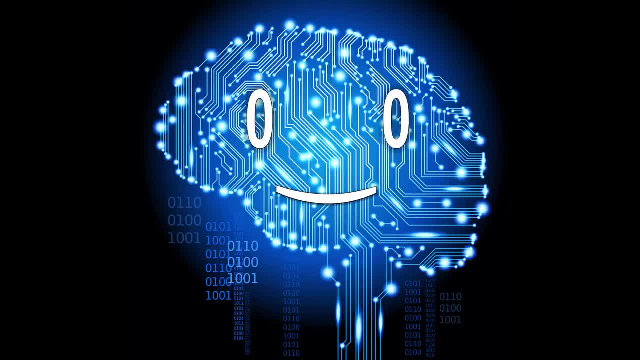 microscope and see what's going on. I don't know what the f**k is this? don't ask me to explain it. As I said, they appear on a very small scale, called the Planck scale, and we are not able to look. 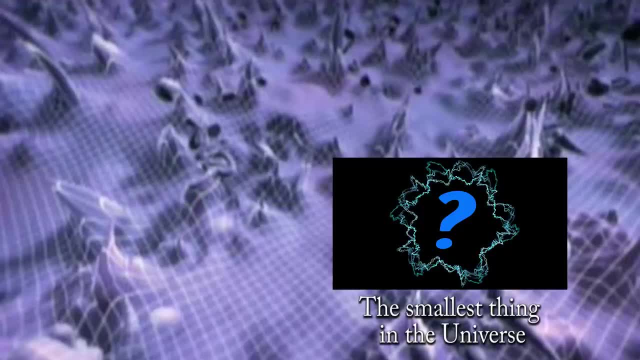 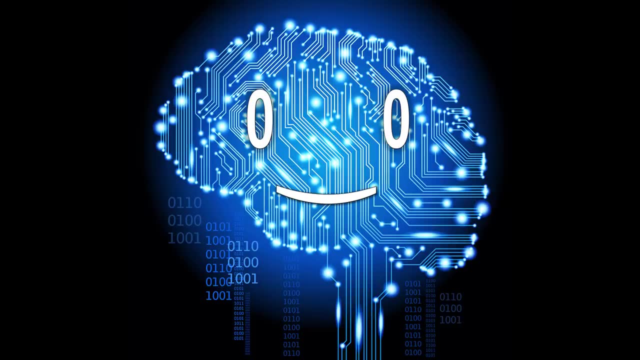 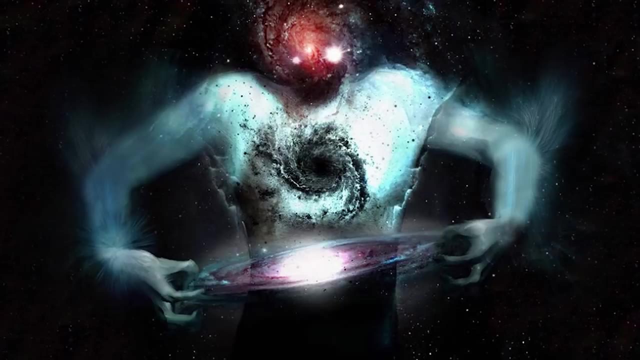 so deep in the fabric of the space. Check out this other video explaining the Planck distance. So yeah, if the existence of the eleven dimensions turns out to be true, we would be able to build wormholes, black holes and meet God. Well, not really, but it would still be pretty awesome. 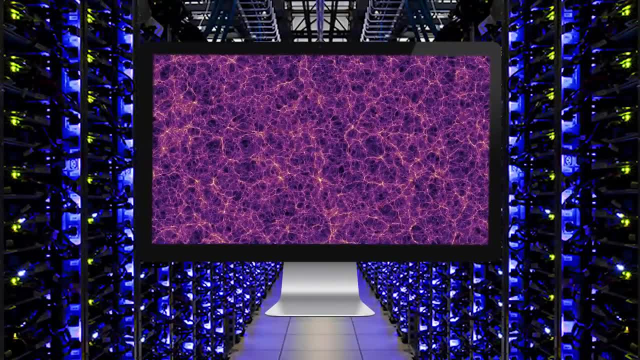 Ah, poor simulations, thinking that there is a purpose to it all.